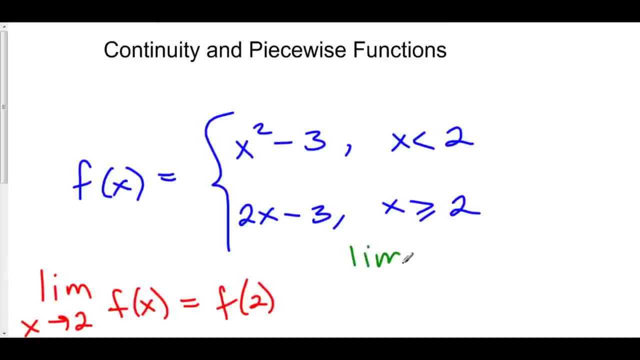 So let's check our left hand limit, The limit as x approaches 2 from the left hand side. well, if we approach 2 from the left hand side, we want x to be less than 2.. We're using x squared minus 3.. This is the function that we're writing to the left of 2.. So here we. 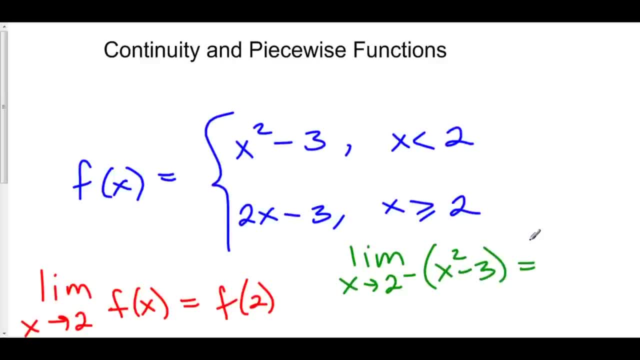 have x squared minus 3.. And of course, step 1 of taking limits is just plug it in: 2 squared is 4 minus 3 is 1.. Boom, All right, Let's check to the right hand side of x equals 2.. So let's check as x approaches 2 from the 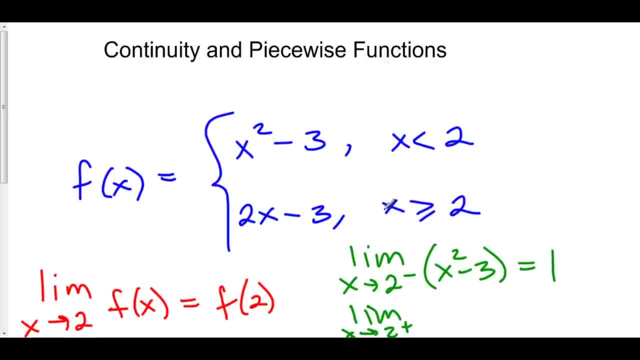 right hand side. From the right hand side, we want x to be bigger than 2.. We're writing our bottom function because that's when x is bigger than 2.. So we're going to check out 2x minus 3.. As we approach 2 from the right hand side of 2x minus 3, we can use our 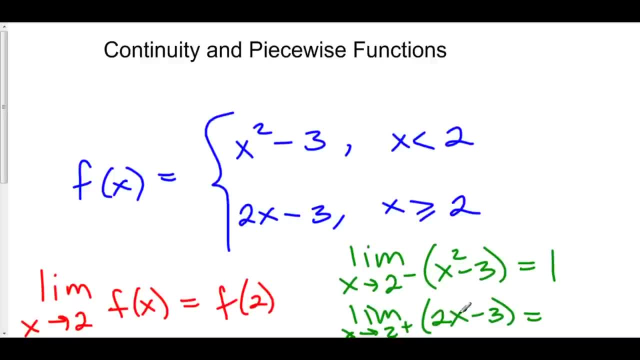 steps to take limits. Step 1. 2 times 2 is 4 minus 3 is 1.. So the limit exists and is 1.. Well, let's check the function value at x equals 2.. Which function are we using at x equals 2?? Well, the one that says: 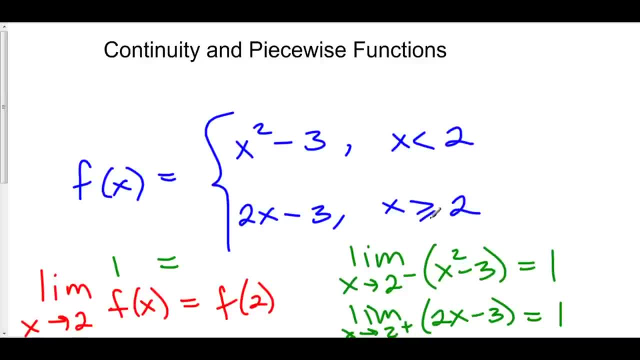 x is greater than or equal to 2.. At x equals 2, we're using our bottom function 2x minus 3.. And if we were to plug 2 into 2x minus 3, we get 4 minus 3 is 2x minus 3.. Well, that's. 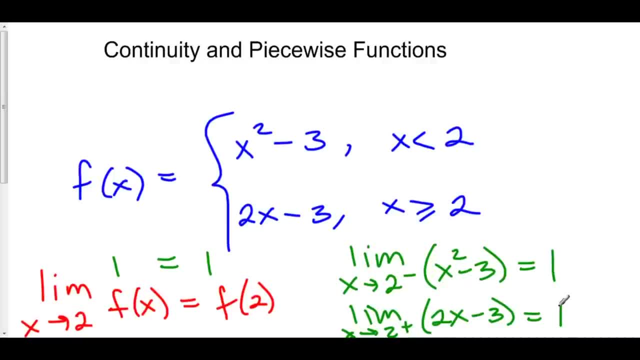 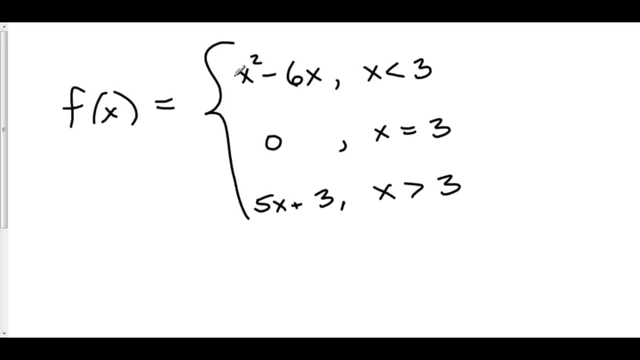 3 times 3 is 1.. So our limit is 1.. The function value is 1. And therefore this function is continuous everywhere, including x equals 2.. Let's check another one Here we have a left hand side where x is less than 3. We have 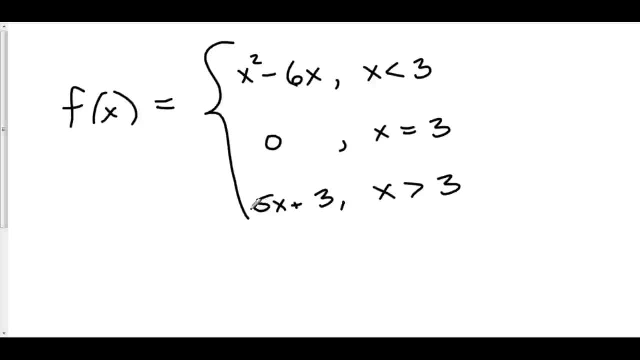 something going on at x equals 3.. And we have something happening from the right hand side of x equals 3.. So Let's first check 1.. Let's first check our limit. We know that x squared minus 6x is continuous everywhere. 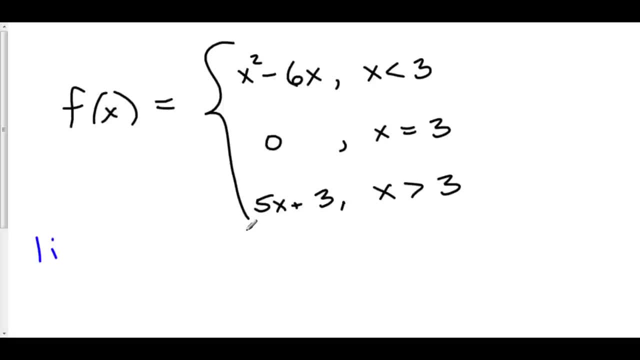 0 is continuous everywhere, And 5x plus 3 is continuous everywhere. So now it comes down to checking our Frankenstein point, Which in this case is 3.. So let's take the limit as x approaches 3 from the left hand side of f of x. Well, if 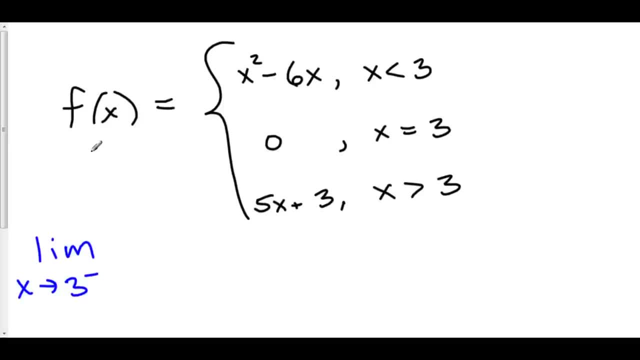 we're approaching 3 from the left hand side. we want to come from the negative side of 3.. From the left of 3. That means that we're going to be using our top. So here we have x squared minus 6x. Step one of finding limits: Plug it in 3 squared. 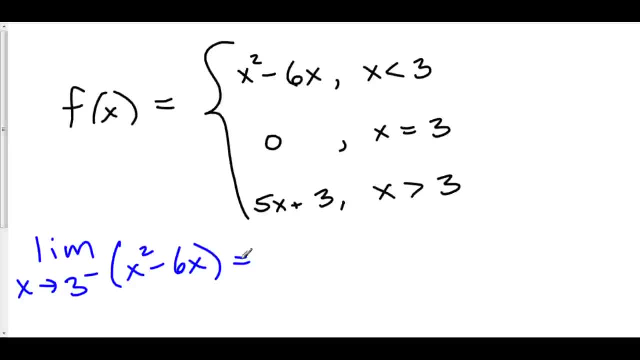 is 9.. Minus 6 times 3 is 18.. 9 minus 18 is negative 9.. Alright, Well, the limit from the left hand side is negative 9.. Let's check the limit from the right hand side. 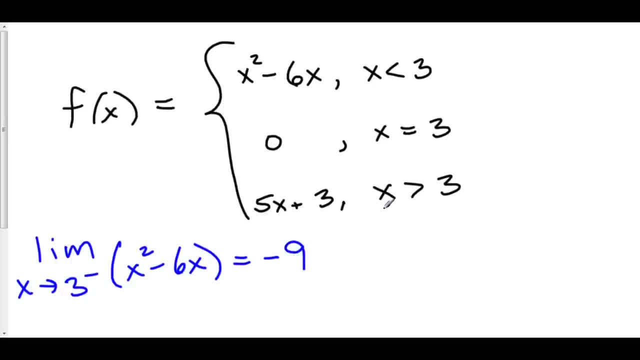 As we approach from the right hand side, we're going from when x is bigger than 3.. So we'll use our bottom function, The limit. as x approaches 3 from the right hand side, we're using 5x plus 3.. Well, 5 times 3 is 15 plus 3 is 18.. Uh oh, the limit doesn't exist. Furthermore, 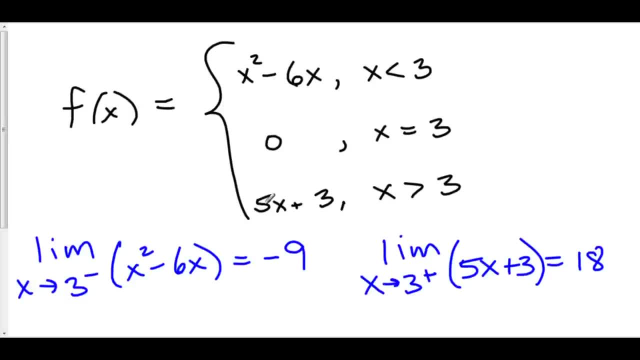 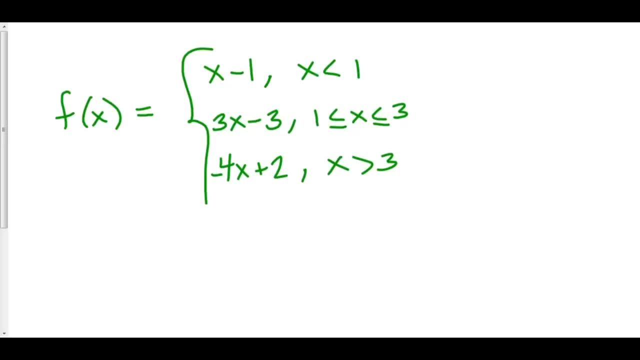 at x equals 3, our function value is 0.. Well, just the fact that our limit doesn't exist means that this is not continuous at x equals 3.. So this is not continuous at x equals 3.. Let's take a look at one more. Here we have two Frankenstein points, One at x equals. 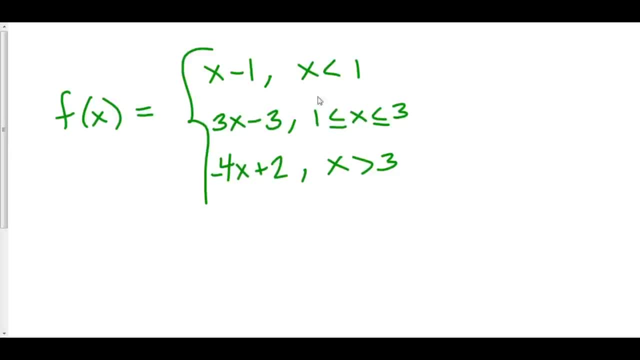 1 and one at x equals 3.. To the left of 1, we're using x minus 1.. From 1 to 3, we're using 3x minus 3, and to the right of 3, we're using negative 4x plus 2.. So let's take a. 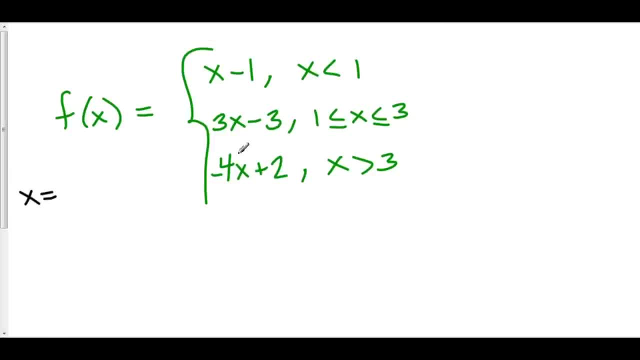 break this apart. Let's check first our first Frankenstein point. x equals 1, because all three of these functions by themselves are continuous. So we'll check the Frankenstein point to see when we put them together if anything weird happens. So the limit as: